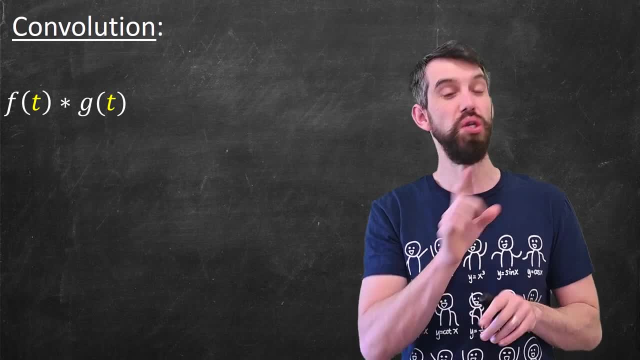 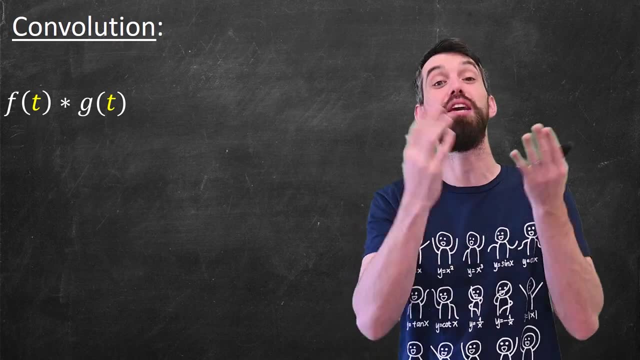 the function g of t. This star that I have here is not the same thing as multiplication. This is a new operation, something new that takes two different functions and combines them to give a third function. The way this is defined might seem at first kind of weird. It's defined to be: 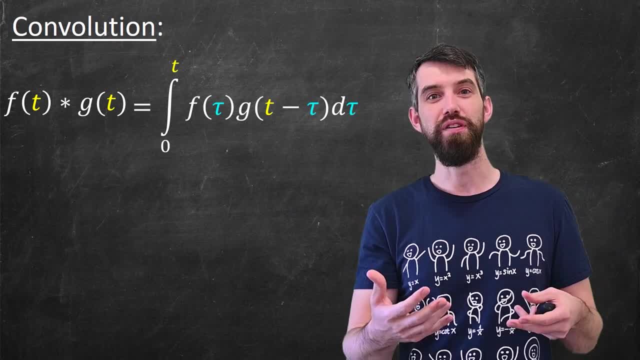 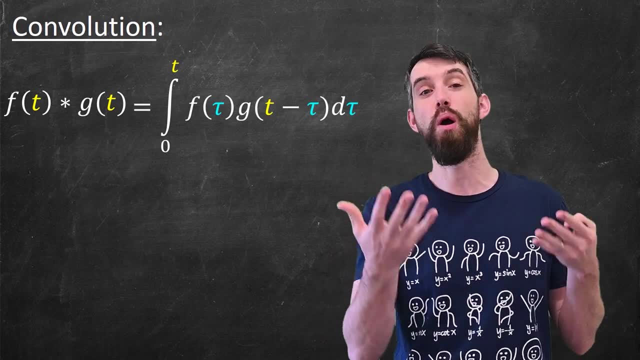 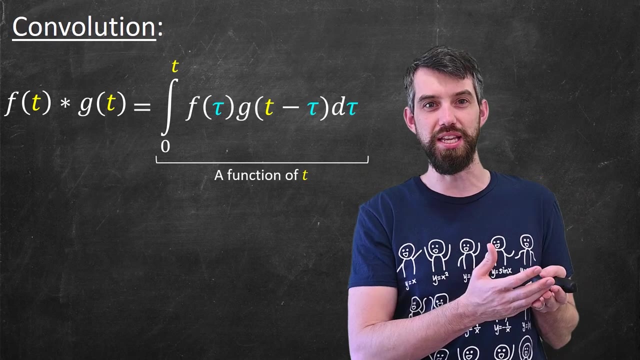 this particular integral. It's an integral from 0 up to t of f, of tau, tau being a dummy. variable integration times, g of t minus tau, and then all integrated with respect to tau. If I look at this right-hand side, well, all of this together is just some function of t: The taus are integrated. 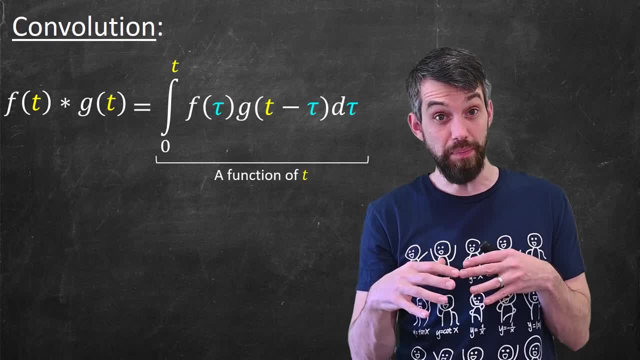 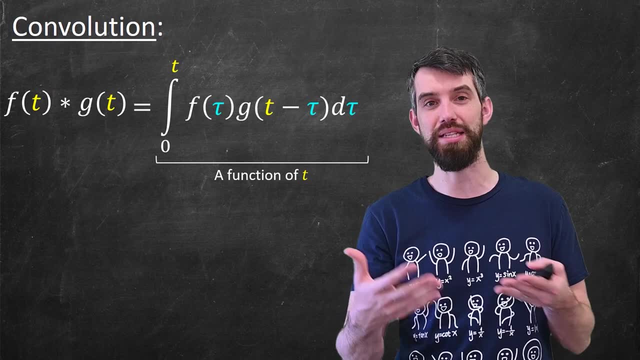 out and that there is a t first inside of the g, but also secondly in the limit of integrations, integral from 0 up to t. So there's two different places that t remain and nevertheless it's a function of t, As long as I presume that my f and my g are actually able to be integrated. 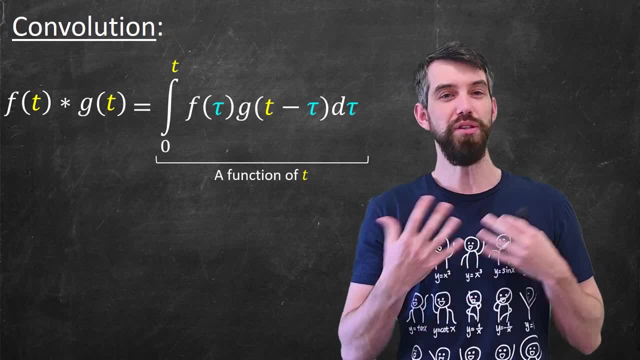 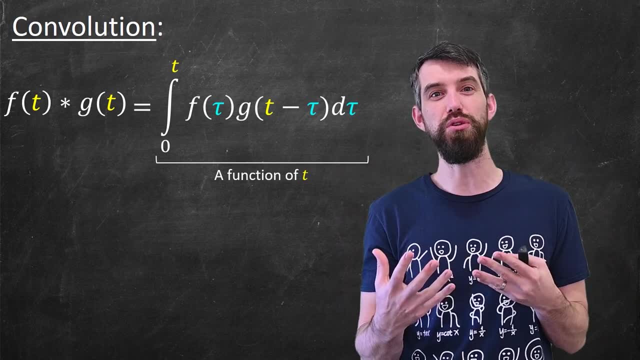 then I have this nice object called the convolution. Now, in this video I'm not going to describe why I might have thought to consider this particular object, but I want to study its properties and see how it's going to be so useful to us. nevertheless, And indeed any time I come, 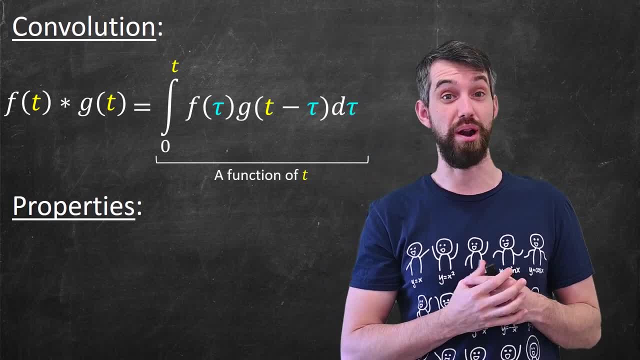 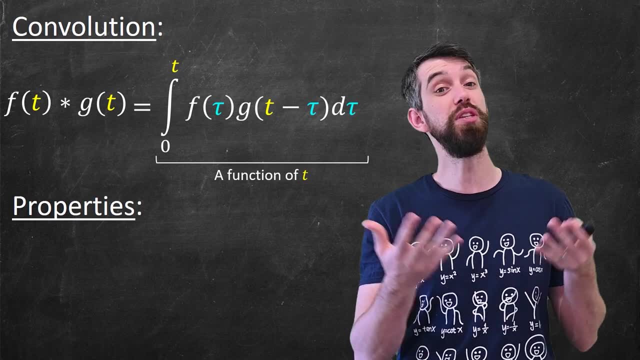 up with a new operation. for example, maybe in linear algebra you figure out how to do matrix multiplication. you should ask: well, what kind of properties does that new operation have? This one has several. The first is that it plays nicely when you interchange the order. It has a. 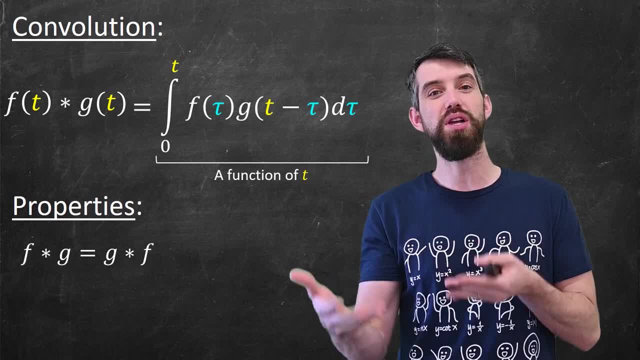 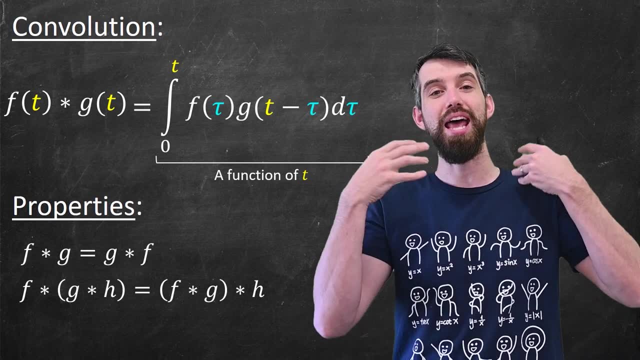 distributivity property, that the convolution of f and g is the same thing as the convolution of g and f. We're going to prove this property in a moment, but let me state the second one, which is going to be an associativity property: The convolution of f with the convolution of g. 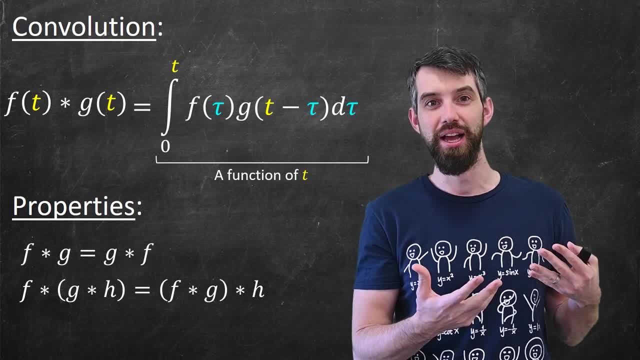 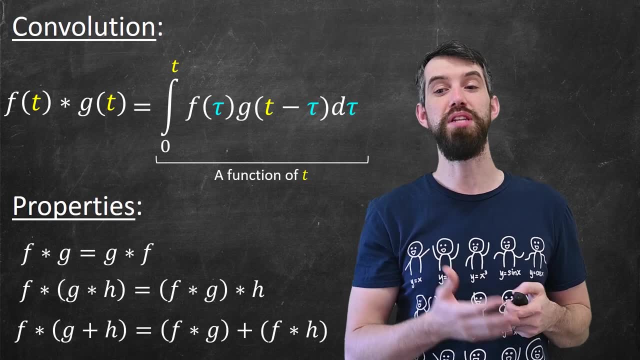 and h is just the same thing as the convolution of f and g, and then you take the convolution of that with h itself. That is an associativity property. And then, finally, we also have a distributivity property, which is that convolutions and normal additions. 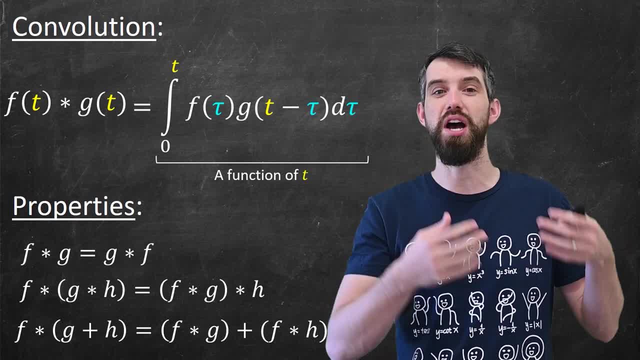 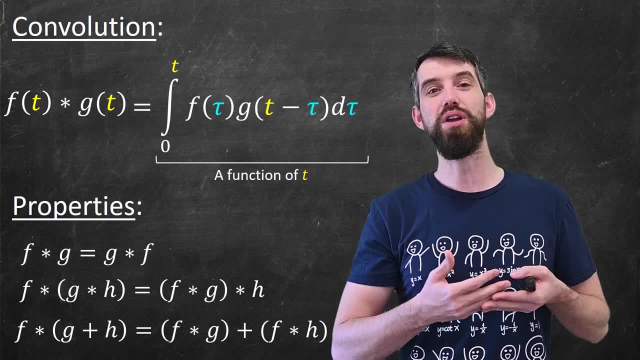 of functions also play well together. So if you take the convolution of the sum of two things, you can distribute the convolution, as they say, over the addition of functions and you get the convolution of f with g and you just add to that the convolution of f with h. I'm just going to 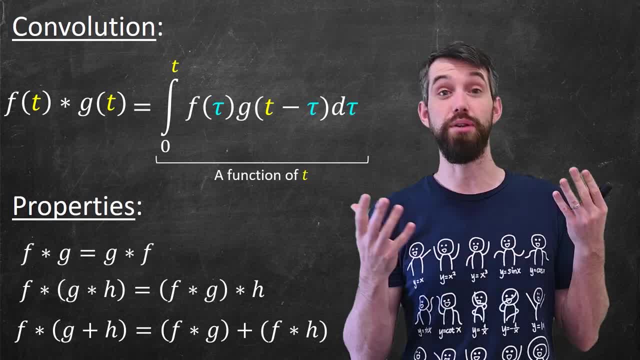 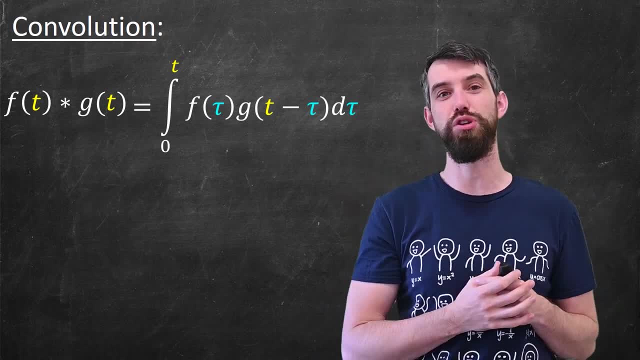 prove the first of these three properties for you, and then I'll leave the second two. as a reasonable exercise, you can pause the video and attempt yourselves. So the first one, the commutivity one. I'm going to begin with the convolution of f of g and I'm going to try to alternate it around. 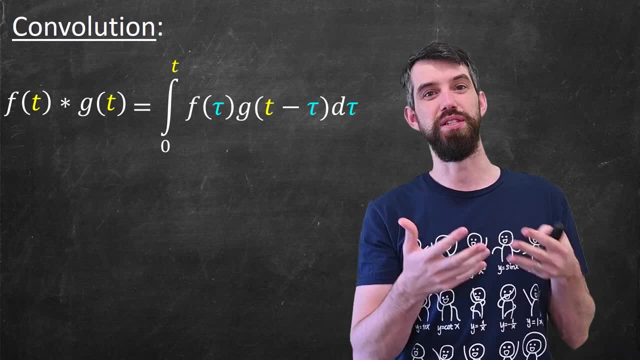 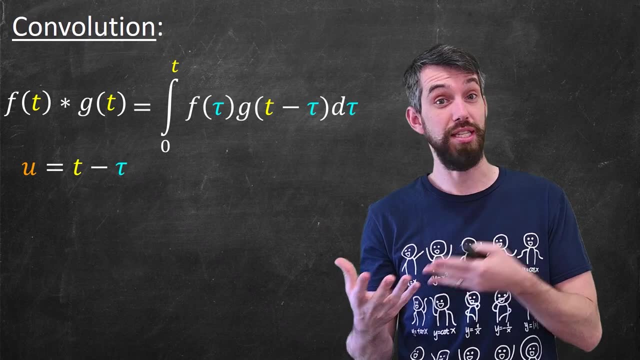 Basically, what I want to do is interchange the role of f and g here, and I'm going to do that. well, just with a substitution. So I'm going to define a new variable, u, which is this difference, this t minus tau. 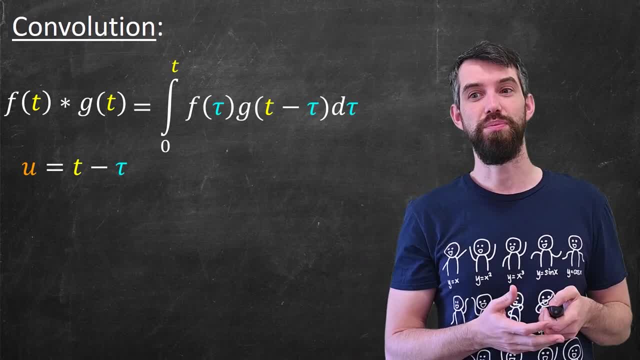 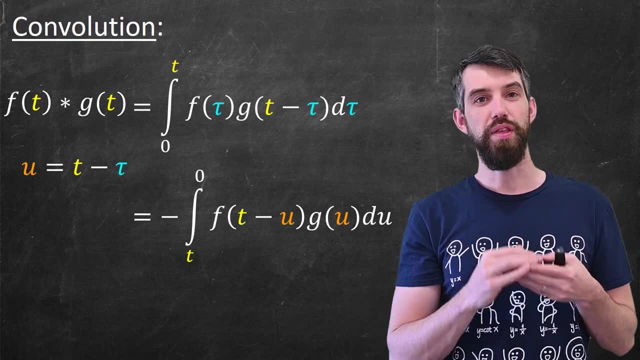 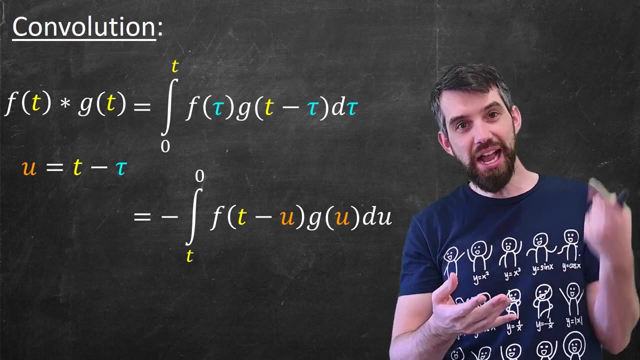 and I'm going to take this change of variables and plug it in. So if I do that, it gives me the following thing: Several things have happened here. The g of t minus tau has turned to a g of u. The f of tau turns into an f of t minus u. The d tau turns into a negative du. That's why the 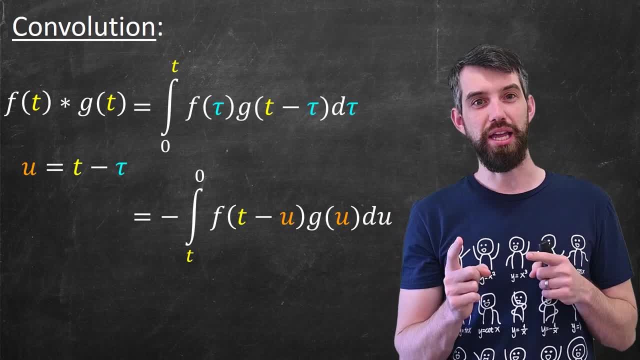 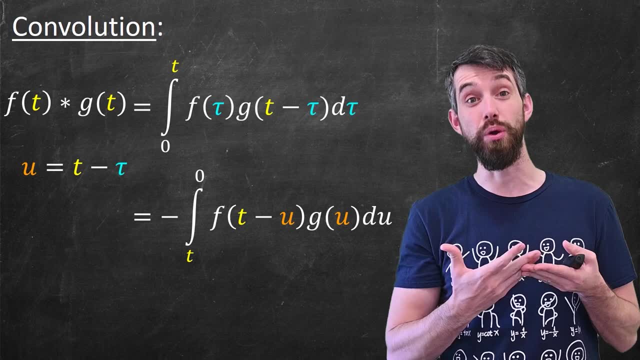 space line, şimdi chi, and we kind of plug it in here. This is a pretty obvious solution. Then, finally, limits of integration change. If you plug in tau equal to 0, you're going to get U equal to t, and if you plug in tau equal to t, you're going to get U equal to 0. So that's. 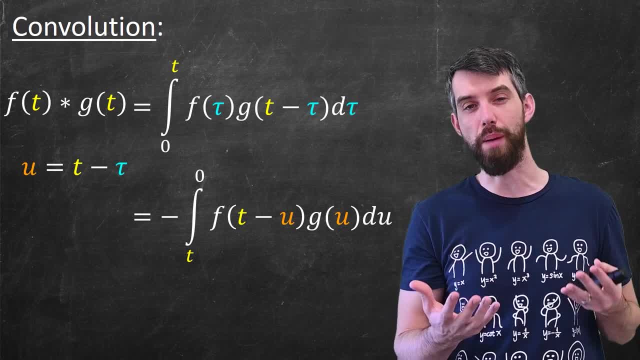 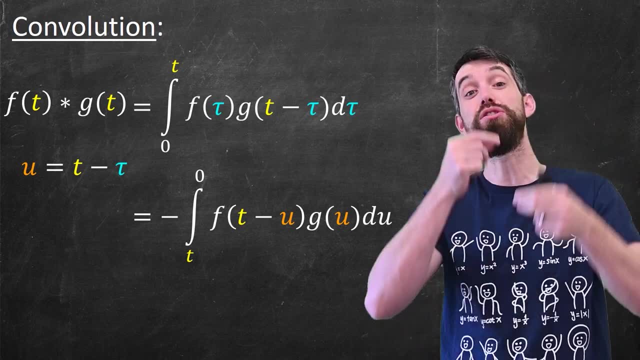 why we have these limits of integrations going from t on the bottom to 0 on the top. It's interchangeable, Okay, so what can I do? Well, I see there's a negative out the front, and so I can use a negative to interchange the limits of integration. so doing that is. 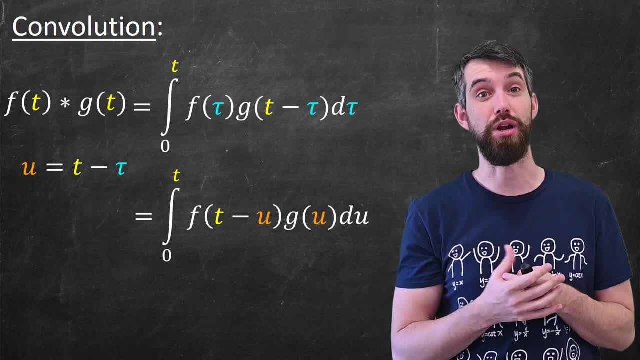 just going to give me the integral from zero up to t of this expression, And the second thing i'm gonna do is thattz that, x, k. I'm going to look at the input and I'm going to go over the whole prism vector. 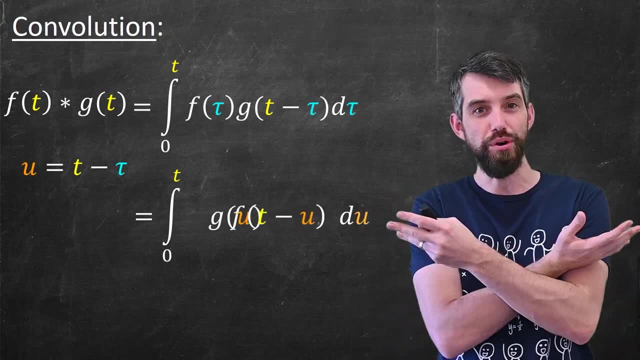 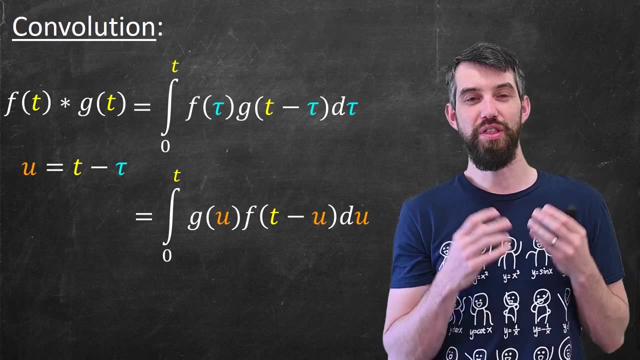 and the second thing I'm going to do is I'm going to alternate the order of the F and the G, just change which comes first, which comes second. and the point is this: with those rearrangements, the integral that I have is now exactly the same as the convolution, but with F and G interchange. that 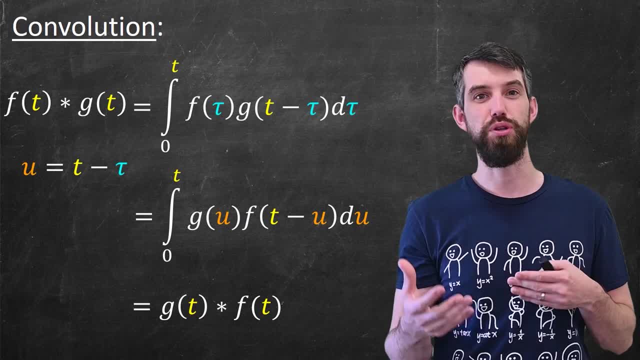 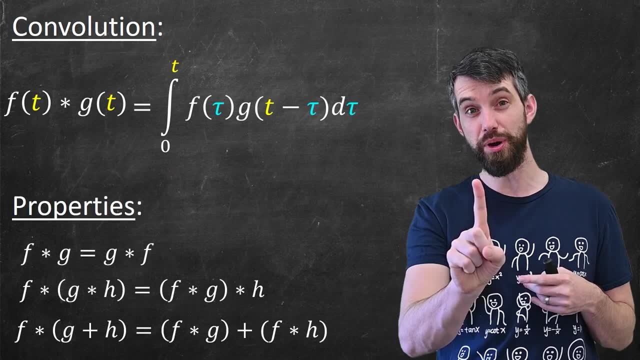 is. this is just the convolution of G with F as opposed to as opposed to the convolution of F with G. nevertheless, we have this cognitivity property. so, as I say, that is the proof of the first property, and then the proofs of the other two properties I'll leave as an exercise for you. 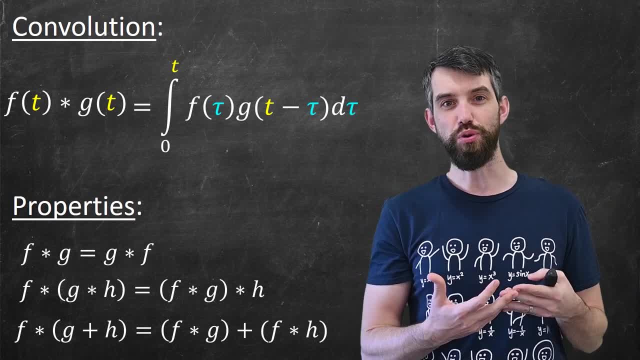 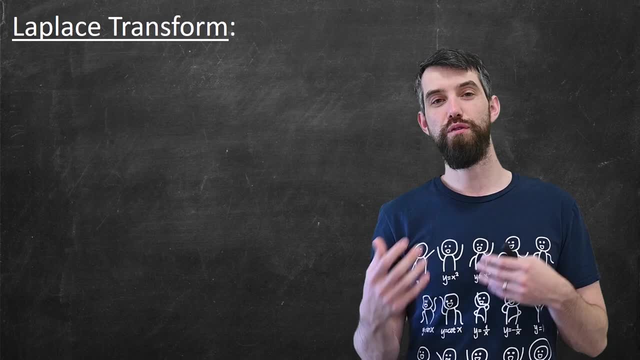 if you wish to pause the video before continuing. the final property is going to be, in some sense, the most important. it's: how do I interact with Laplace transforms? now, before I talk specifically about the convolution, I want to observe that Laplace transforms plays nicely, for example, 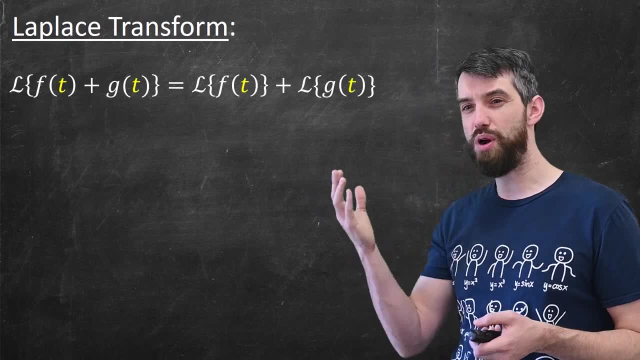 with the addition of functions, there's this sort of linearity property that says that the Laplace transform of a sum is just the sum of two different Laplace transforms. Laplace transform of a sum is just the sum of two different Laplace transforms Laplace transforms. 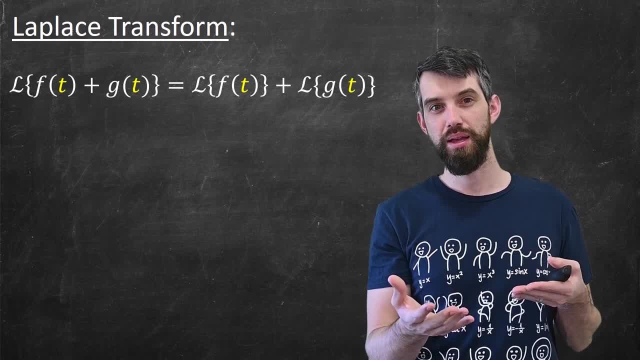 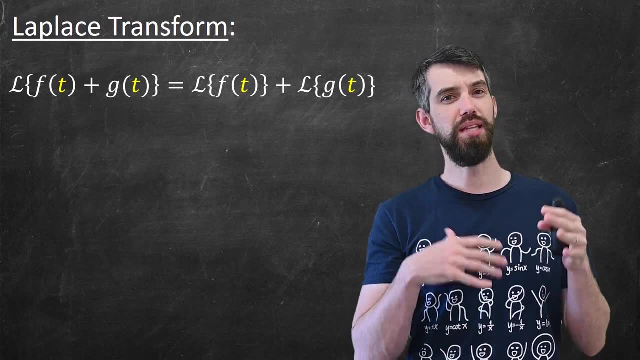 transform of F added to the Laplace transform of G. indeed, if you want to put coefficients A and B in front of those F and G, we also have linearity there as well. however, the same kind of property is definitely not true when it comes to multiplication of functions. that is, you might. 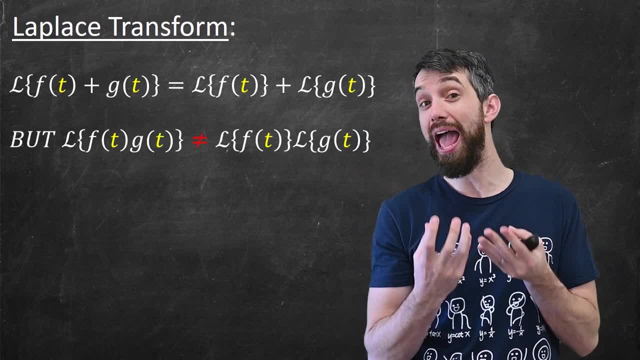 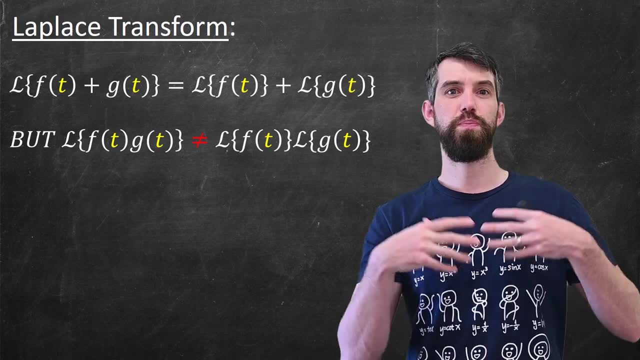 have guessed that if you took the Laplace transform of a multiplication F times G, that that would just be the Laplace transform of F times the Laplace transform of G. but but this is not true. this is perhaps to be expected. we know that the Laplace transform of F times the Laplace 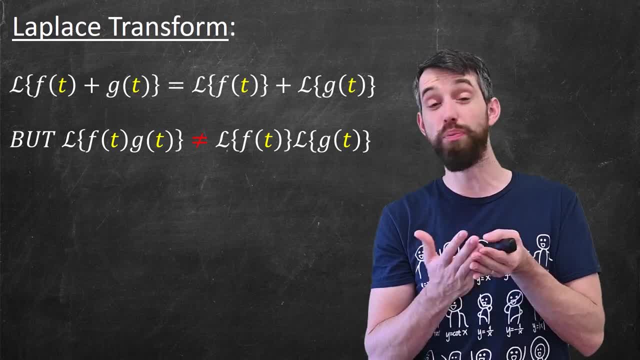 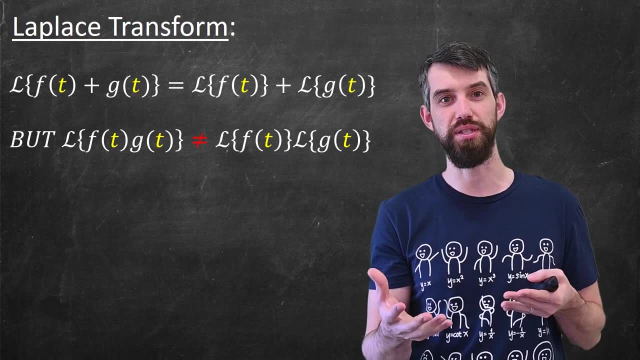 transform of F times the Laplace transform of G is not the derivative of a product, is not the product of the derivative. it obeys the product rule. we know that the integral of a product is likewise not the product of two different integrals. there's the integration by parts formula for that. 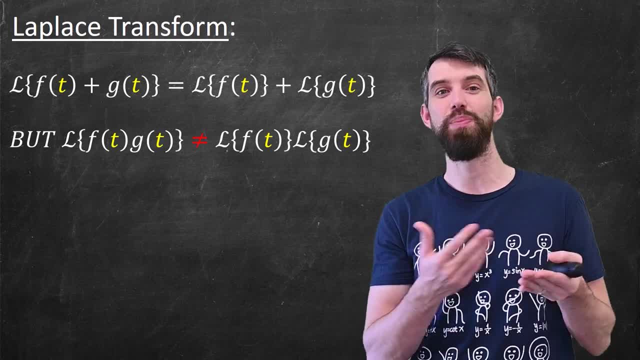 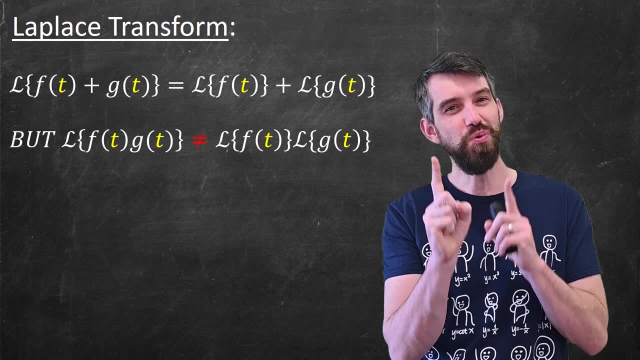 so the point is, we should not have expected the Laplace transform, which is some sort of integral formula, to work out nicely for products, and indeed it doesn't. but it does work out nicely for convolutions, that is, if instead of F times G I take the Laplace transform of F times G. 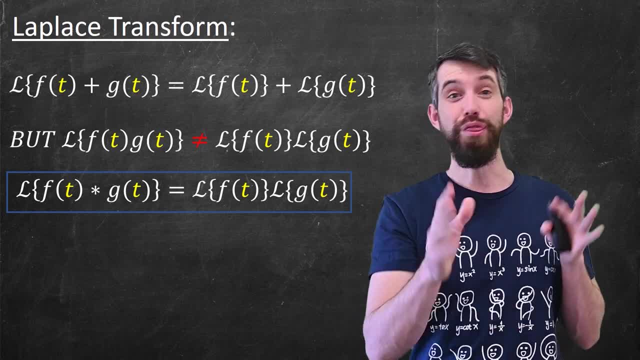 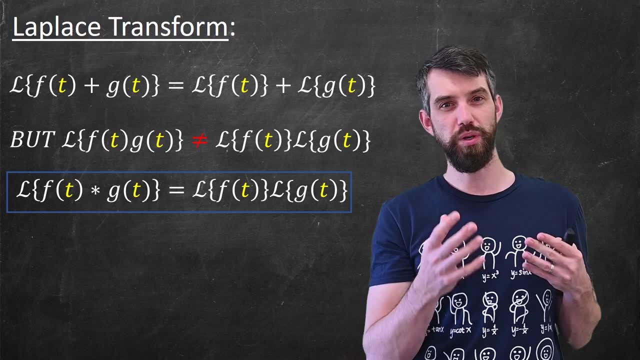 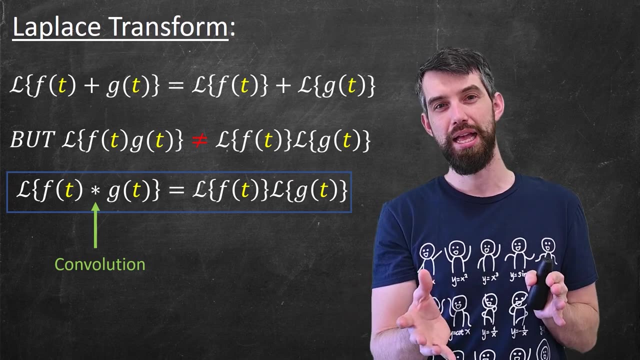 then it is just going to be the Laplace transform of F multiplied by the Laplace transform of G. so it's worth noting that there's really two different operations here. there's this star which we use to denote convolution, that particular integral, and then there's also 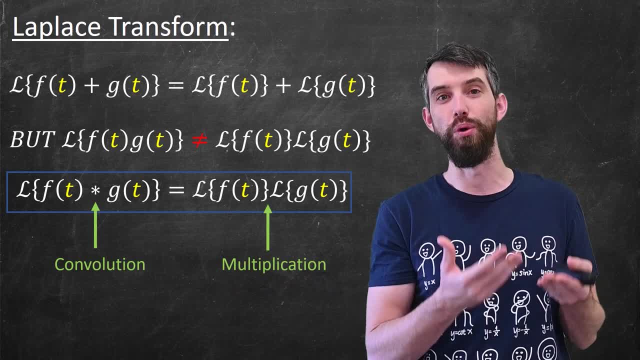 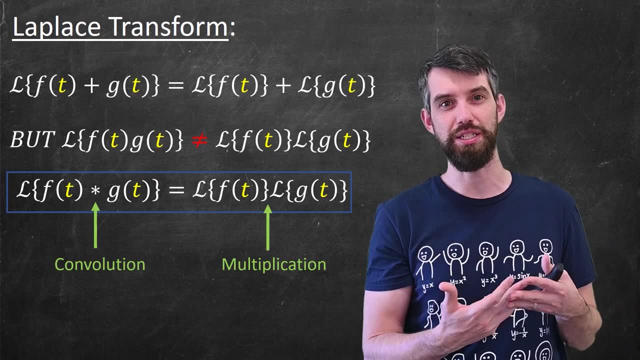 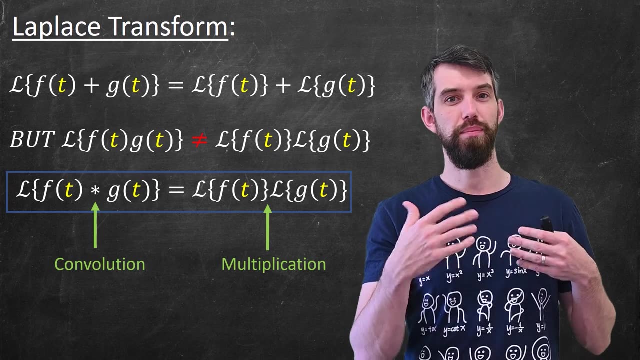 juxtaposition which we use to denote just normal old multiplication, like two times three is six. so the right side of this expression is just normal multiplications of functions, where the left-hand side involves the convolution of two functions. this new and more complicated operation, I might wish to use the standard names that the Laplace transform of little f is big F of s and 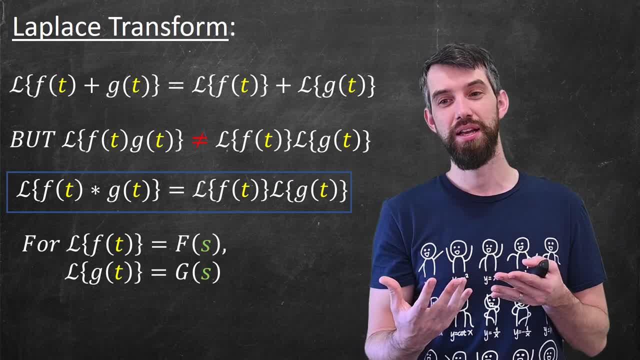 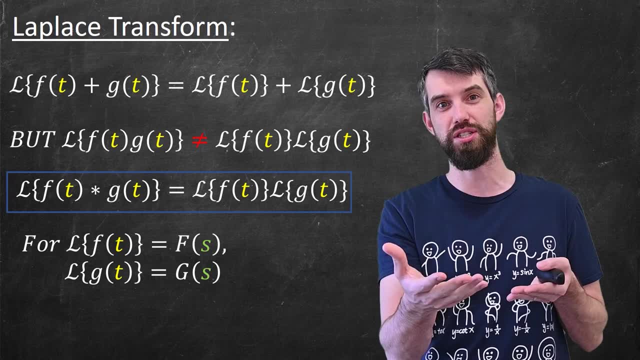 likewise, the Laplace transform of little g is big G of s. in that case, the formula would read that the Laplace transform of little f convoluted with little g is just going to be equal to big F times big G, and this is perhaps best stated when I actually am asking, not. 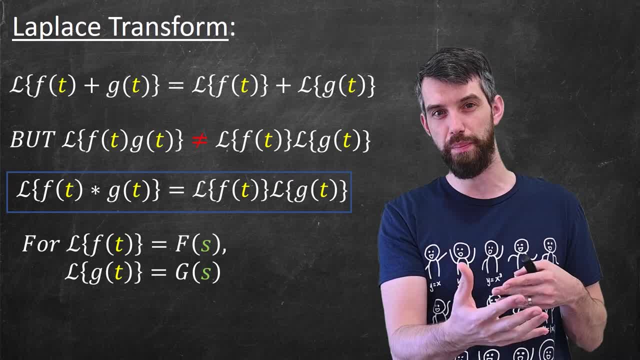 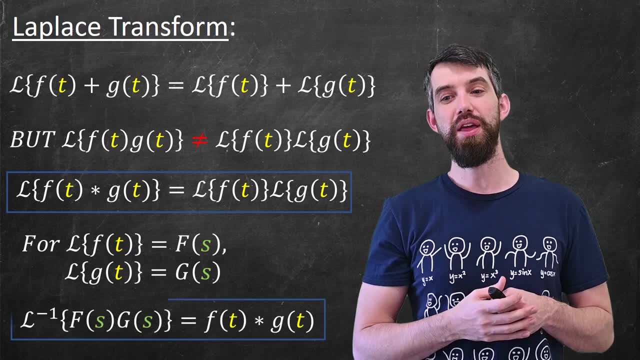 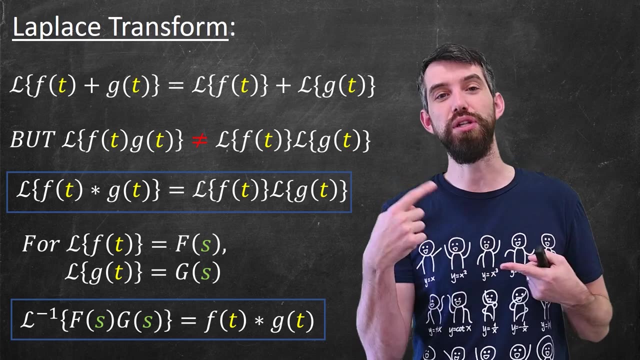 about the Laplace transform, but the inverse Laplace transform. that is, if I take this statement and go the other way around and apply the inverse Laplace transform to it, then well, the inverse Laplace transform of a multiplication of functions is therefore going to be the convolution of the little f and the little g. the inverse Laplace transforms of: 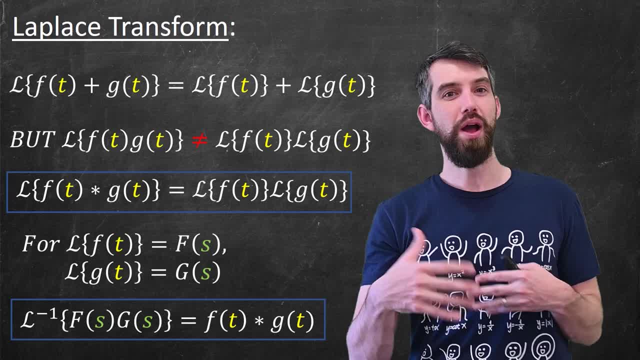 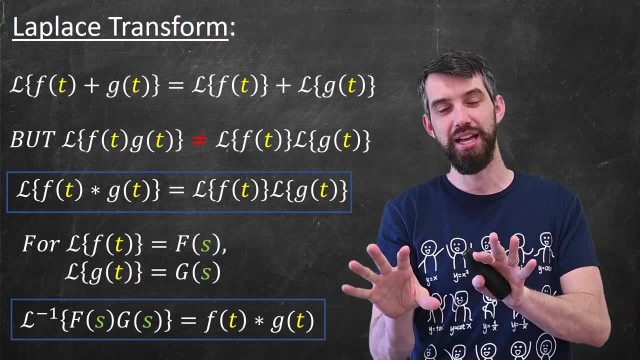 the big F and the big G respectively. the reason why it's so nice in this form is that if you're using the Laplace transform to solve a differential equation, and somewhere you get a product, the big challenge is trying to find the inverse Laplace transform. 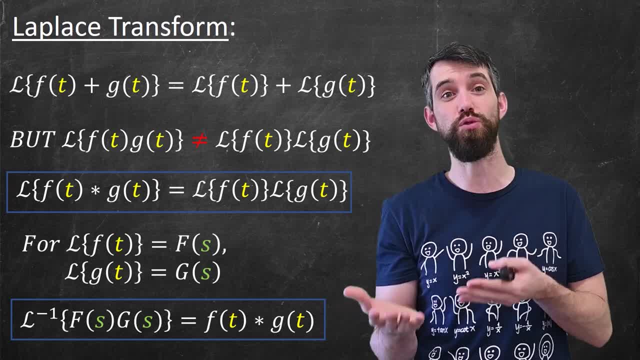 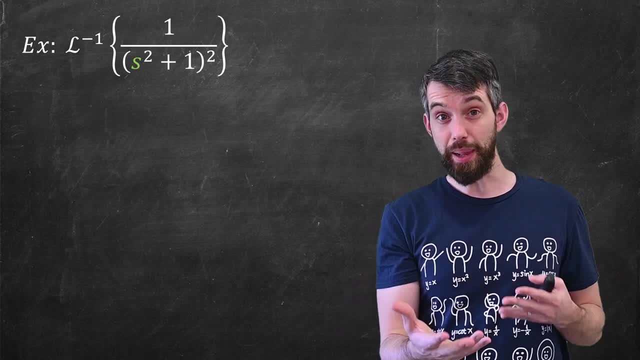 But now I know how to find the inverse Laplace transform of a product. well, it's going to be this convolution, All right. so let's see an example. Here I'm asking to find the inverse Laplace transform of this particular function. 1 over. 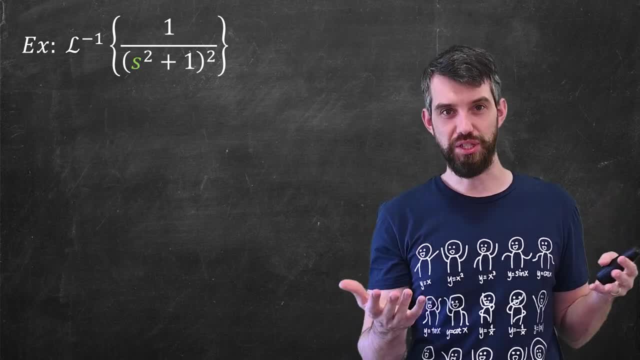 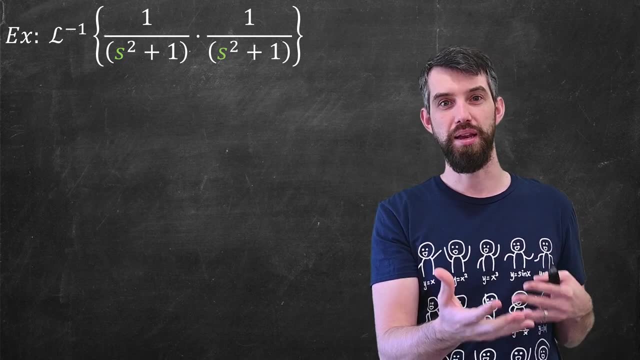 s squared plus 1, all squared, And perhaps the first thing I'll do is just sort of rearrange it to more explicitly look like the product of two different functions, Namely there's 1 over s squared plus 1, and then multiplies. another copy of that. 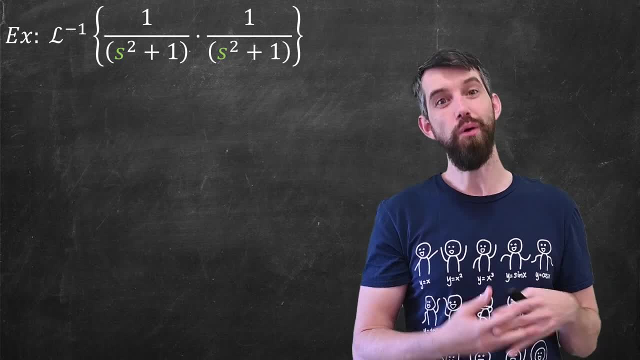 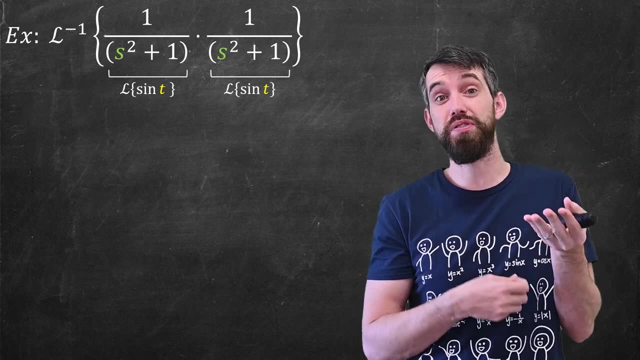 Now, these two different factors that are being multiplied are ones that I hopefully recognize That individually they look like the Laplace transform of sine. they're both the same, So it looks like I've got the Laplace transform of sine multiplied by another copy of the 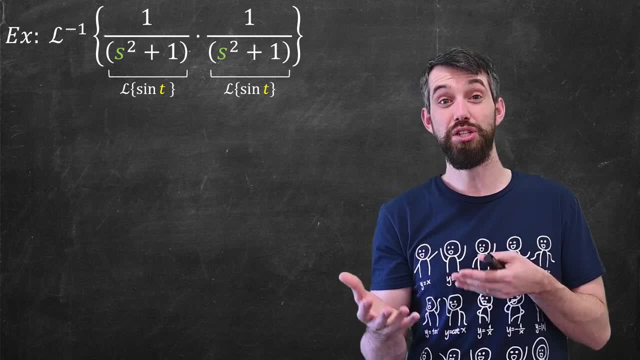 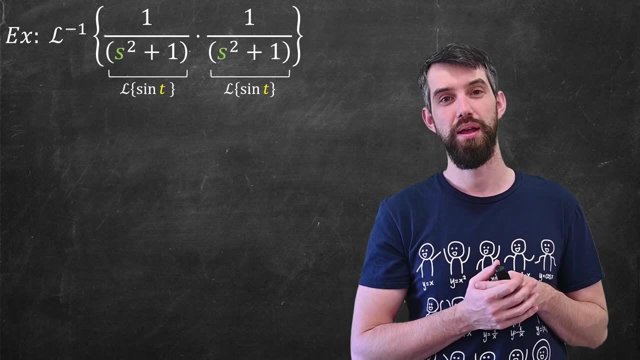 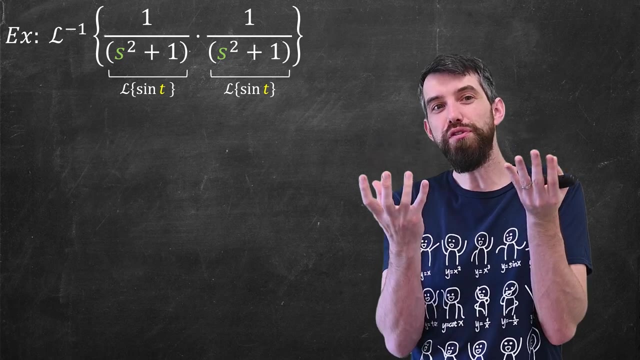 Laplace transform of sine. Now, as mentioned, the Laplace transform of a product is not just the product of Laplace transform. so the answer to this is not just sine squared, as much as we might wish it to be. what we've just seen is that the inverse Laplace transform of a product is the convolution of the 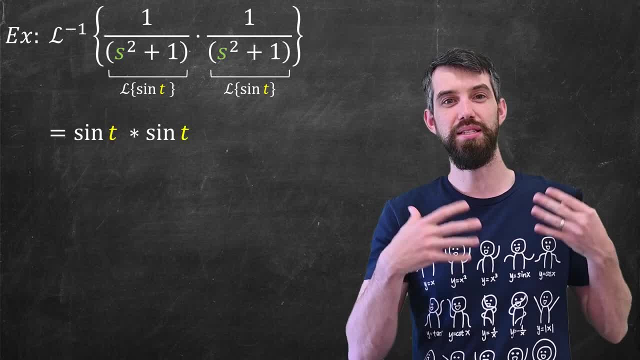 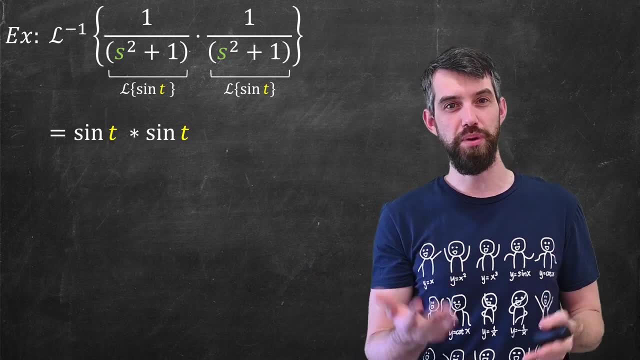 inverse Laplace transform of the two different factors, That is, this is sine of t convoluted with sine of t again. Okay, well, now I have something that I actually can compute, because the convolution is a defined thing. It's this particular integral, the integral from 0 to t. 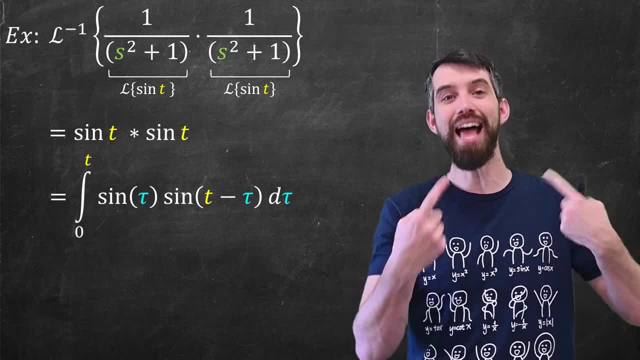 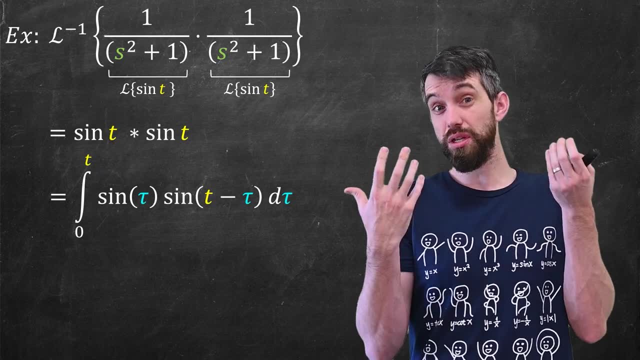 We'll take the first function sine, write sine of tau. We'll take the second function, sine and write now sine of t minus tau and integrate all this out with respect to tau. And so now it's just a computational question. It's a question of: do we know how to compute?